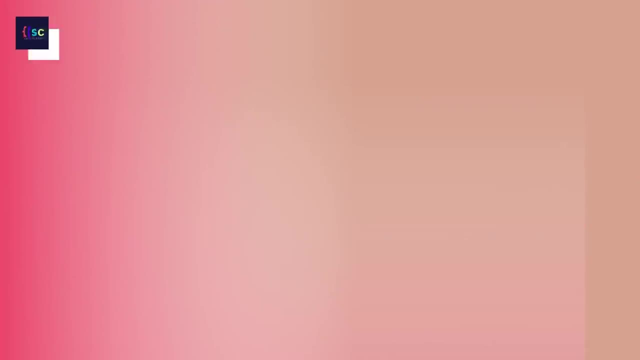 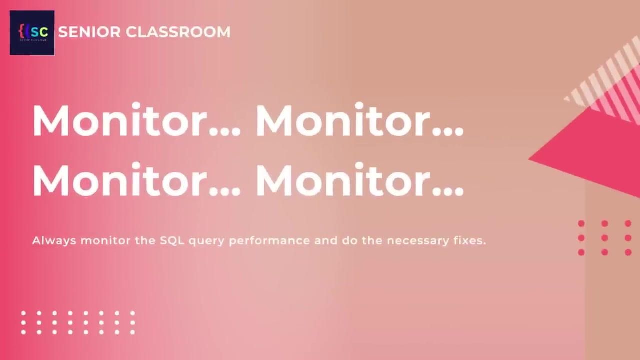 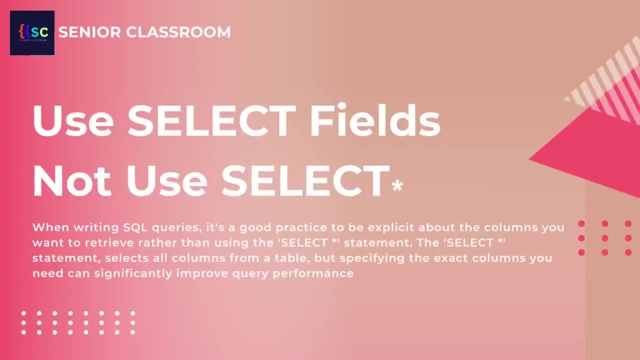 that subscribe button and ring the notification bell so you won't miss any of our future content. Now let's get started. First technique is always specify select fields. Avoid select star statement. When writing SQL queries, it's a good practice to be explicit about the columns you want to retrieve, rather 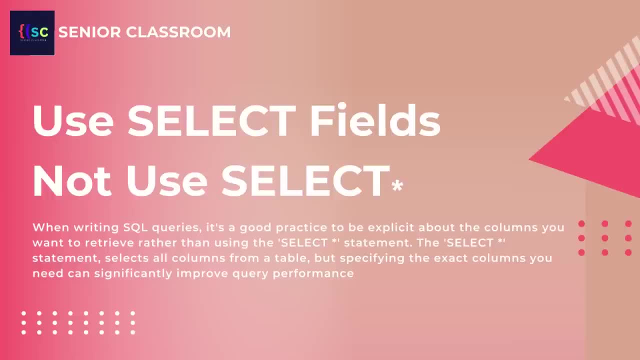 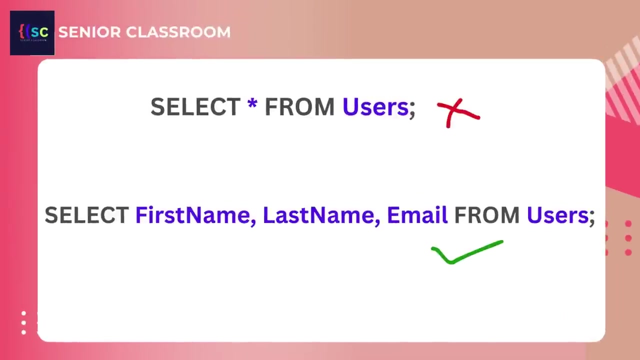 than using the select star statement. The select star statement selects all columns from a table, but specifying the exact columns you need can significantly improve query performance. Selecting only the necessary columns reduces the amount of data transferred between the database and the application, improving query speed. It minimizes 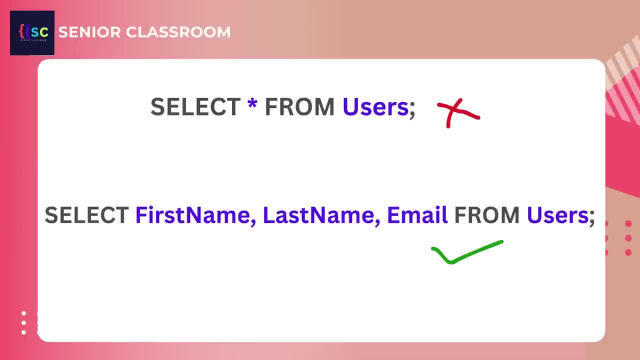 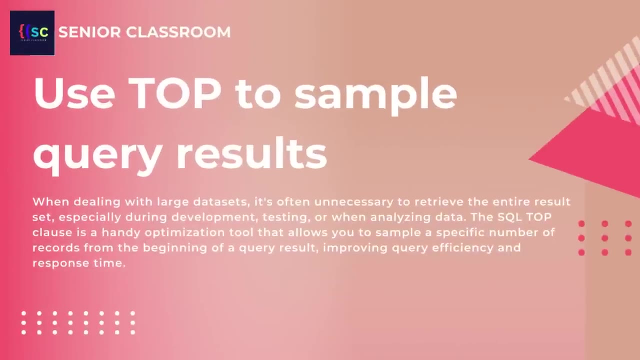 the workload on the database server by fetching only the required data, resulting in faster query execution times. Next is use top to sample query records. When dealing with large data sets, it's often unnecessary to retrieve the entire results set, especially during development, testing or when analyzing data. The SQL top. 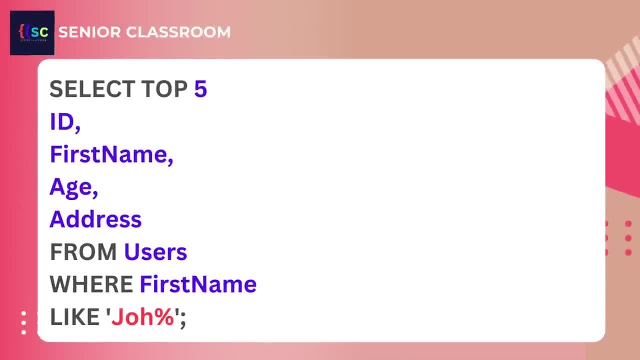 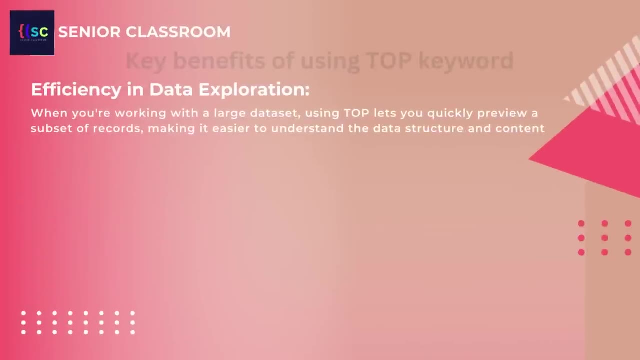 clause is a handy optimization tool that allows you to sample a specific number of records from the beginning of a query result, improving query efficiency and response time. Key benefits are efficiency in data exploration When working with a large data set. using TOP lets you quickly preview a subset of records making. 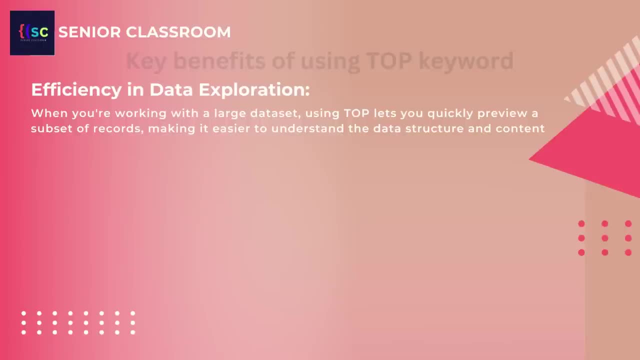 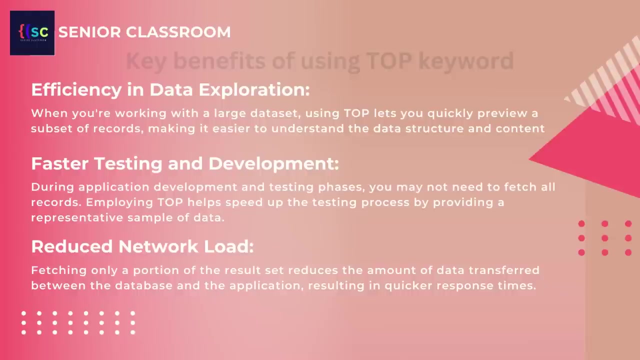 it easier to understand the data structure and content. Faster testing and development. During application development and testing phases, you may not need to fetch all records. Employing TOP helps speed up the testing process by providing a representative sample of data. Increased network load. Fetching only a portion of the result set reduces the amount of data. 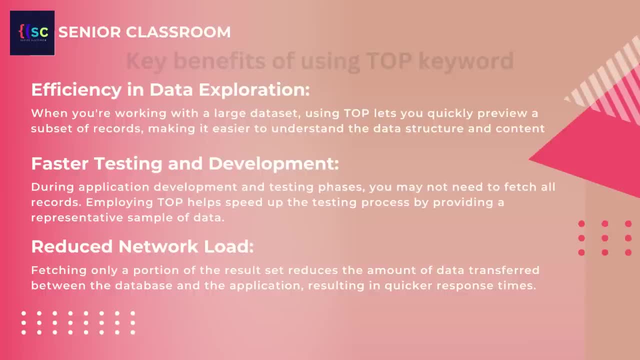 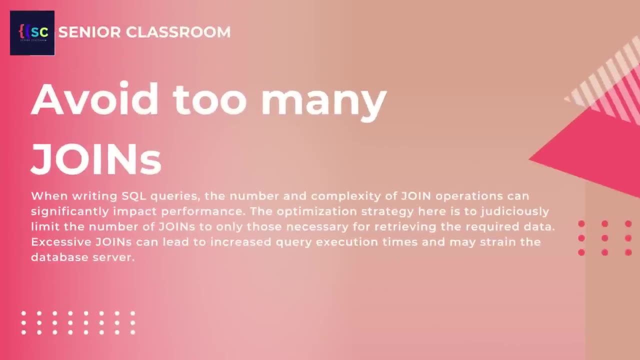 transferred between the database and the application, resulting in quicker response times. Next is avoid too many joins When writing SQL queries. the number and complexity of join operations can significantly impact performance. The optimization strategy here is to judiciously limit the number of joins and reduce the number of joins. 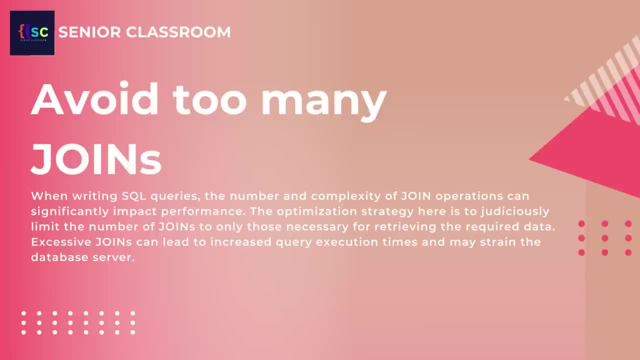 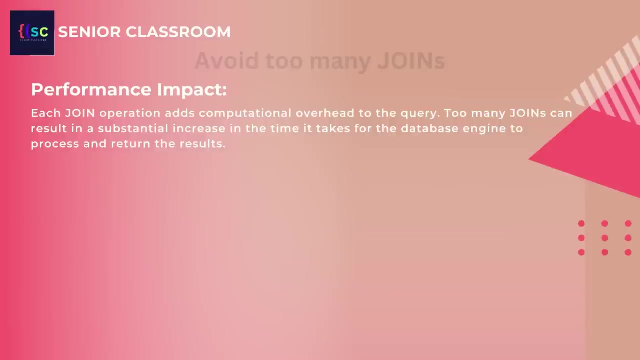 to only those necessary for retrieving the required data. Excessive joins can lead to increased query execution times and may strain the database server. Key considerations are: performance impact: Each join operation adds computational overhead to the query. Too many joins can result in a substantial increase in the time it takes. 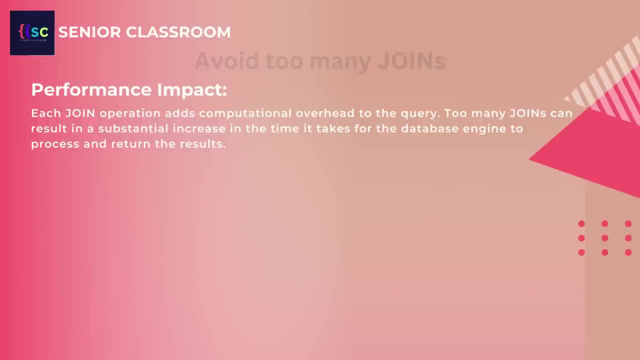 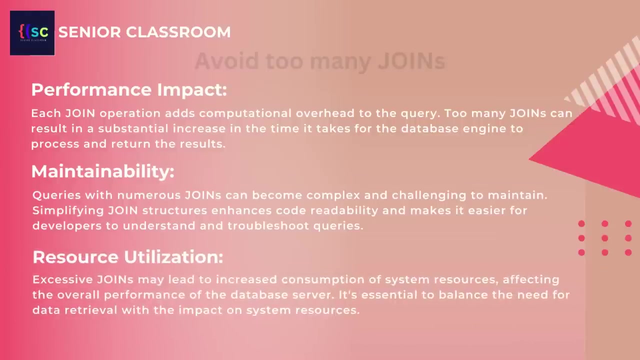 for the database engine to process and return the results. Maintainability: Queries with numerous joins can become complex and challenging to maintain. Simplifying join structures enhances code readability and makes it easier for developers to understand and troubleshoot queries. Resource utilization: Excessive joins may lead to increased consumption of system resources. 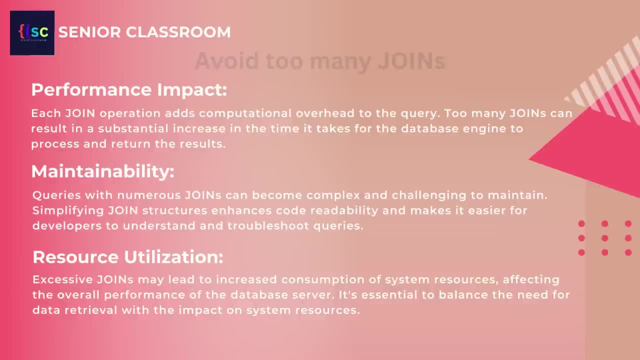 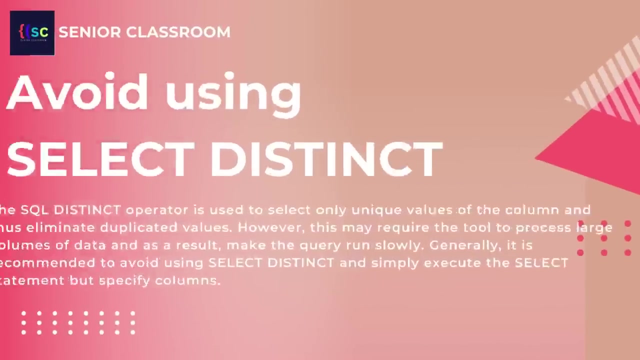 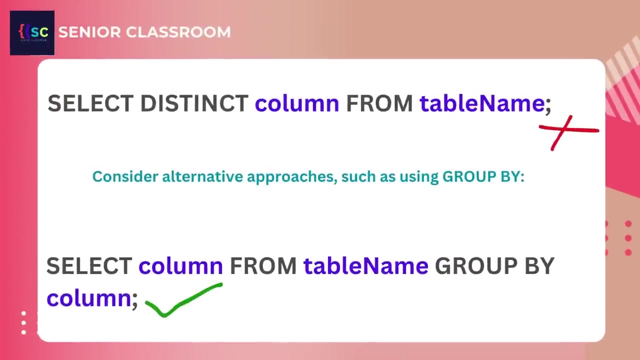 affecting the overall performance of the database server. It's essential to balance the need for data retrieval with the impact on system resources. Next is avoid using Select Distinct. While Select Distinct is a powerful tool for fetching unique values from a column, it can be resource intensive and impact query performance. 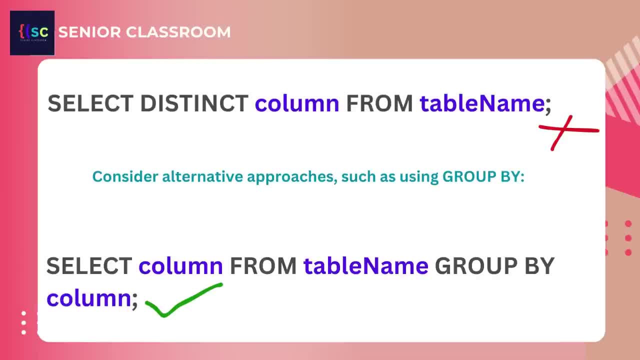 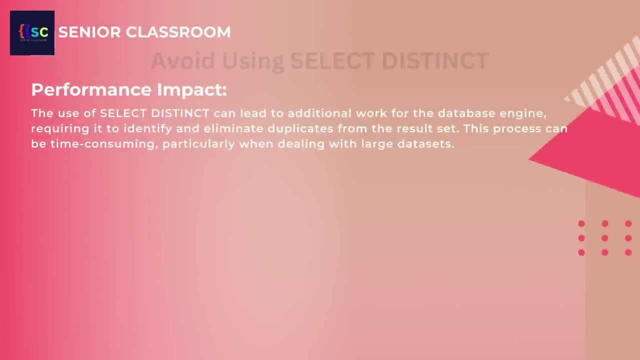 especially when applied to large data sets. The optimization strategy here is to consider alternatives and use the data that is available to you. Use Distinct judiciously to prevent unnecessary processing overhead. Key considerations are performance impact. The use of Select Distinct can lead to additional work for the database engine. 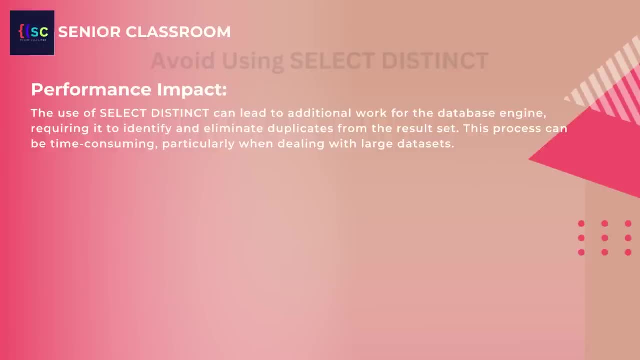 requiring it to identify and eliminate duplicates from the result set. This process can be time-consuming, particularly when dealing with large data sets. Alternative approaches- In some cases, achieving the same results without using Select Distinct- is possible Utilizing Group, By proper indexing or restructuring the query. 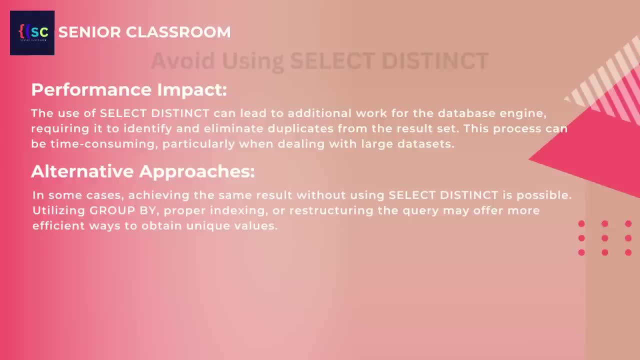 may offer more efficient ways to obtain unique values Resource utilization. Reducing the reliance on Select Distinct can help conserve system resources, ensuring better scalability and improved responsiveness of the database. Next, you can use Select Distinct to reduce the reliance on Select Distinct. 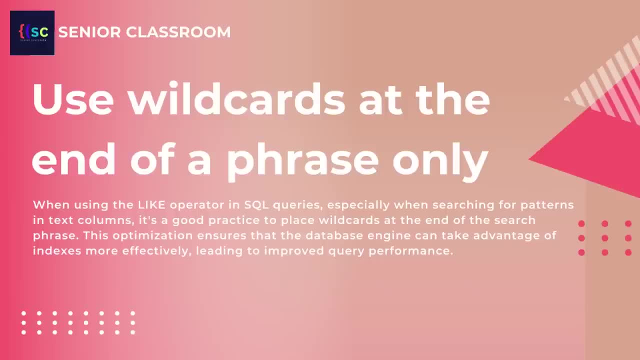 Use Wildcards at the end of a phrase only When using the Like operator in SQL queries. especially when searching for patterns in text columns, it's a good practice to place Wildcards at the end of the search phrase. This optimization ensures that the database engine 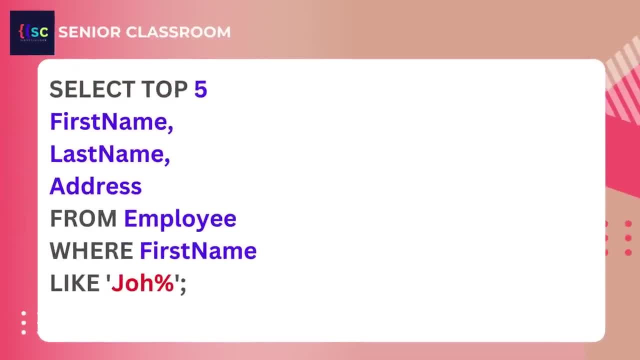 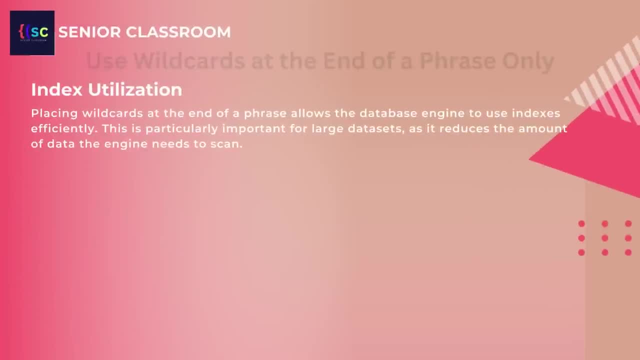 can take advantage of indexes more effectively, leading to improved query performance. Key considerations are: index utilization: placing Wildcards at the end of a phrase allows the database engine to use indexes efficiently. This is particularly important for large data sets, as it reduces the amount of data the engine needs to scan. 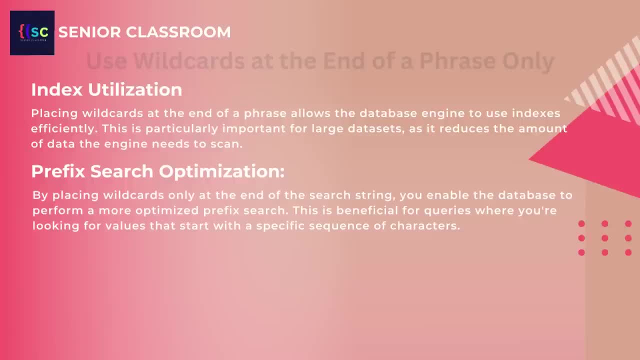 Prefix search optimization. By placing Wildcards only at the end of the search string, you enable the database to perform a more optimized prefix search. This is beneficial for queries where you're looking for values that start with a specific sequence of characters. Performance impact. 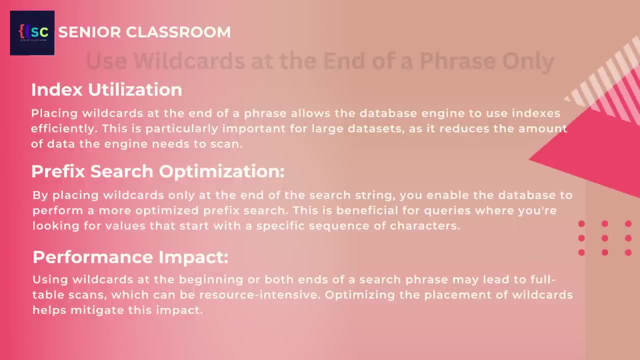 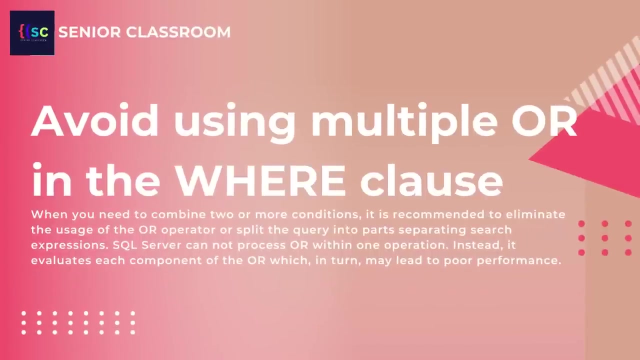 Using Wildcards at the beginning or both ends of a search phrase may lead to full table scans, which can be resource intensive. Optimizing the placement of Wildcards helps mitigate this impact. Next technique is avoid using multiple OR in the WHERE clause When you need to combine two or more conditions. 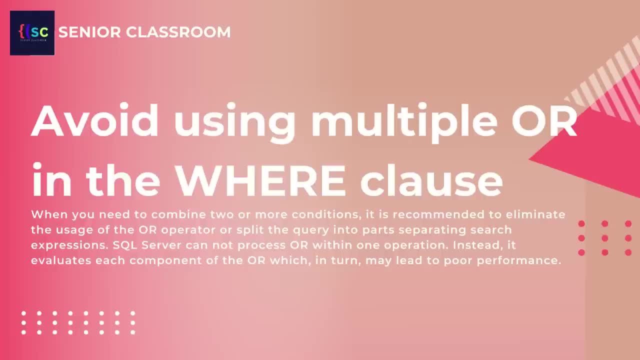 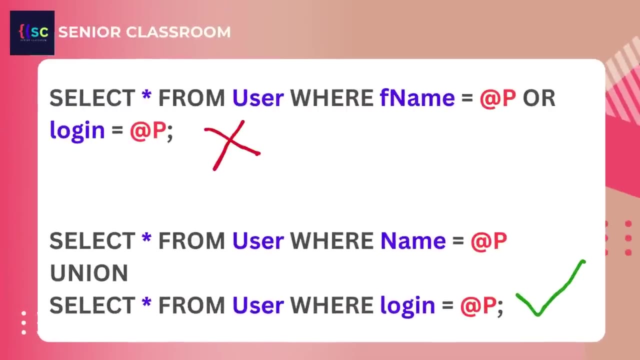 it is recommended to eliminate the usage of the OR operator or split the query into parts separating search expressions. SQL Server cannot process OR within one operation. Instead, it evaluates each component of the OR, which in turn may lead to poor performance. Key considerations are: 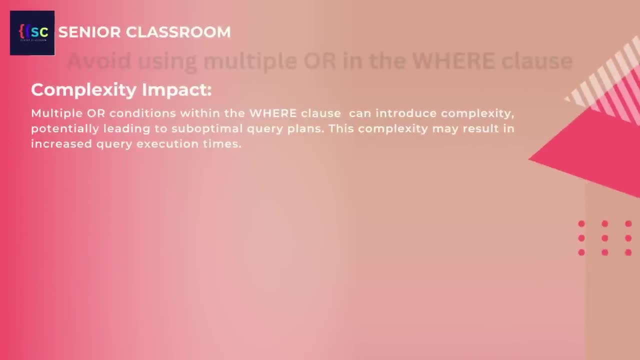 Complexity impact. Multiple OR conditions within the WHERE clause can introduce complexity, potentially leading to suboptimal query plans. This complexity may result in increased query execution times. Index utilization: Complex OR conditions can make it challenging for the database engine to fully utilize indexes. 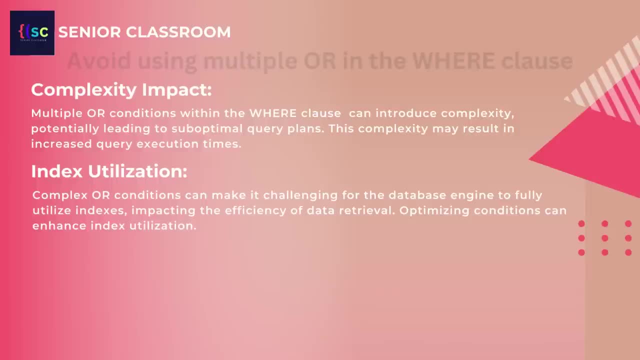 impacting the efficiency of data retrieval. Optimizing conditions can enhance index utilization, Readability and maintainability. Simplifying the WHERE clause improves query readability and maintainability. It makes the code more straightforward, facilitating easier understanding, debugging and future modifications. Next is 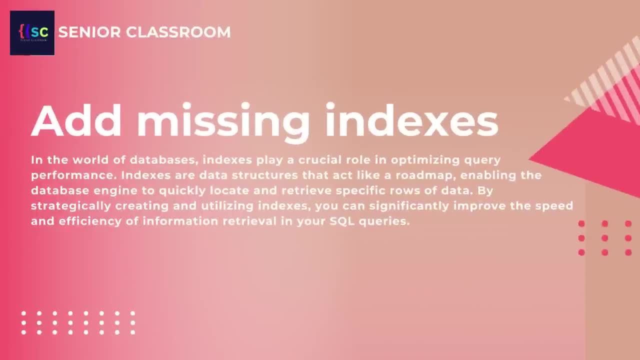 Add missing indexes. In the world of databases, indexes play a crucial role in optimizing query performance. Indexes are data structures that act like a roadmap, Enabling the database engine to quickly locate and retrieve specific rows of data By strategically creating and utilizing indexes. 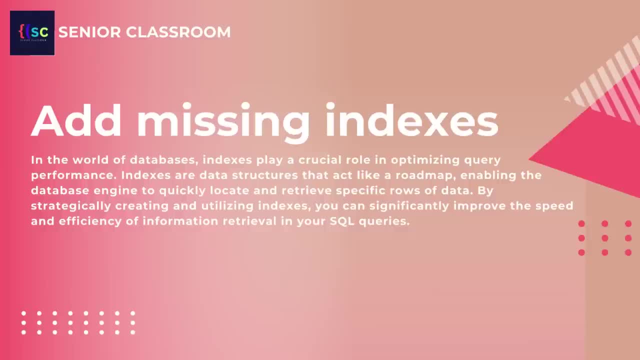 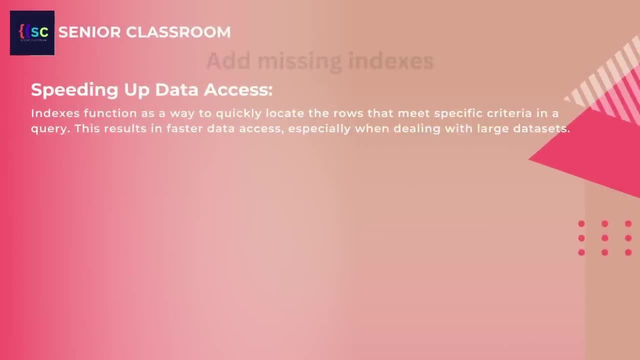 you can significantly improve the speed and efficiency of information retrieval in your SQL queries. Key considerations are: Speeding up data access. Indexes function as a way to quickly locate the rows that meet specific criteria in a query. This results in faster data access. 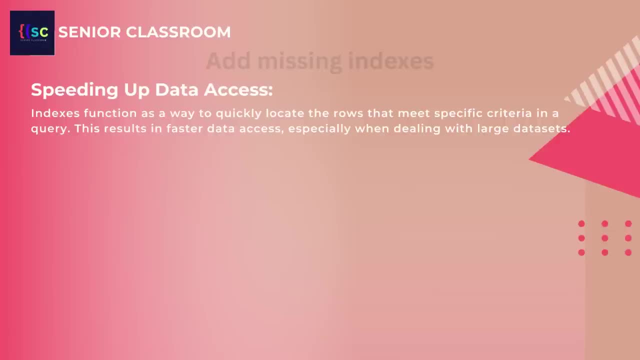 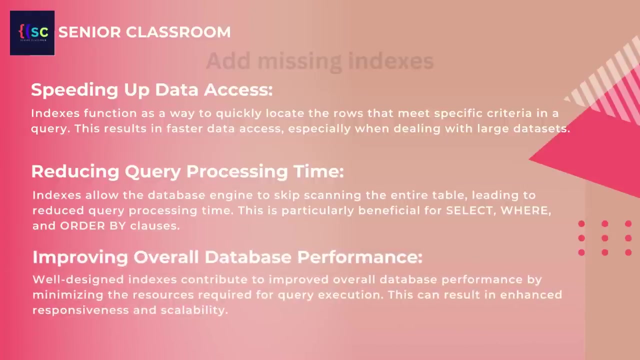 especially when dealing with large data sets. Reducing query processing time. Indexes allow the database engine to skip scanning the entire table, leading to reduced query processing time. This is particularly beneficial for select WHERE and ORDER BY clauses, Improving overall database performance. 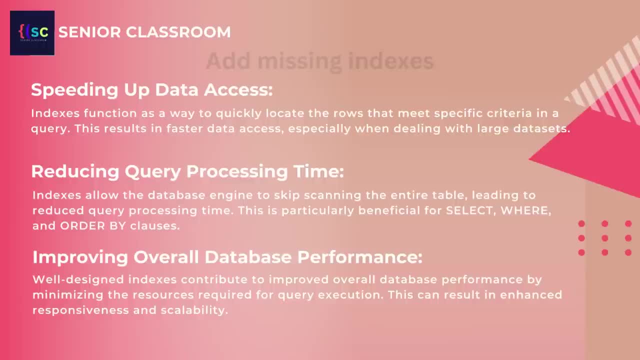 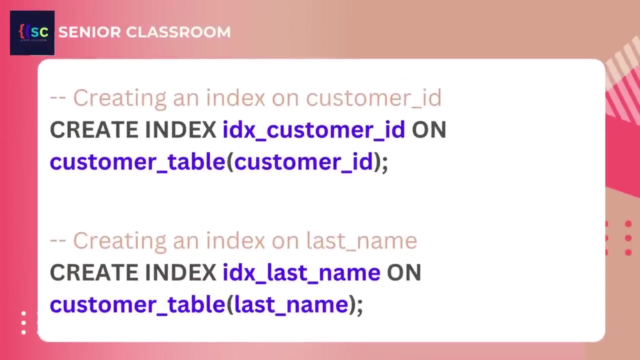 Well-designed indexes contribute to improved overall database performance by minimizing the resources required for query execution. This can result in enhanced responsiveness and scalability. How to apply this technique: Identify key columns. Identify columns frequently used in WHERE clauses, JOIN conditions or ORDER BY statements. 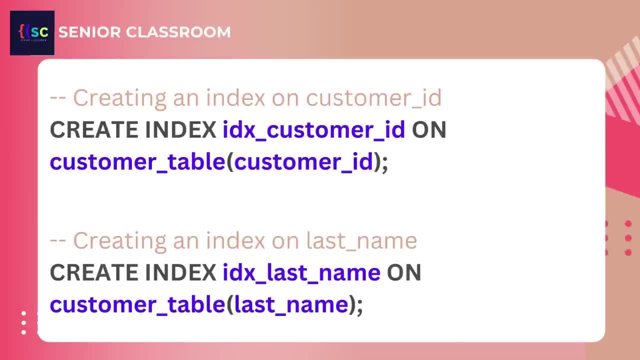 These are often good candidates for indexing. Understand query patterns. Understand the typical patterns of queries executed against your database. Create indexes that align with these patterns to maximize their impact. Consider composite indexes For queries involving multiple columns. consider creating composite indexes that cover those columns. 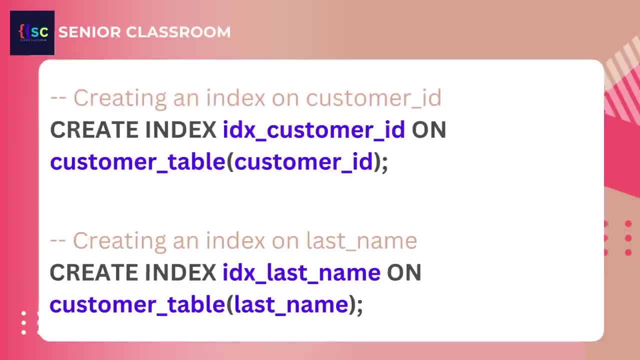 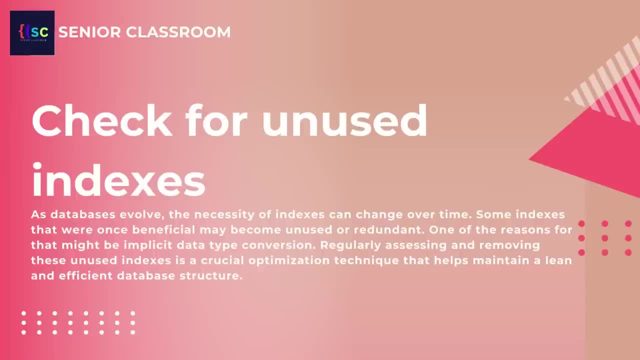 This can further optimize query performance. Next is Check for unused indexes. As databases evolve, the necessity of indexes can change over time. Some indexes that were once beneficial may become unused or redundant. One of the reasons for that might be implicit data type conversion. 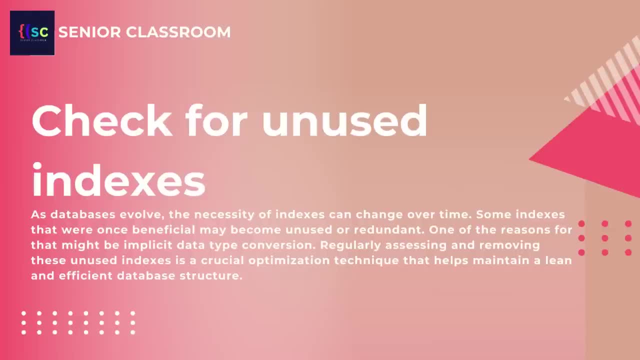 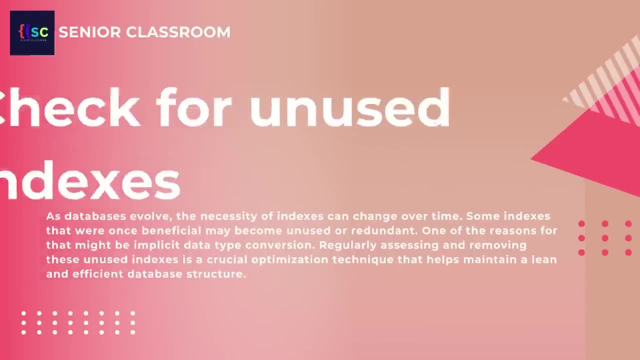 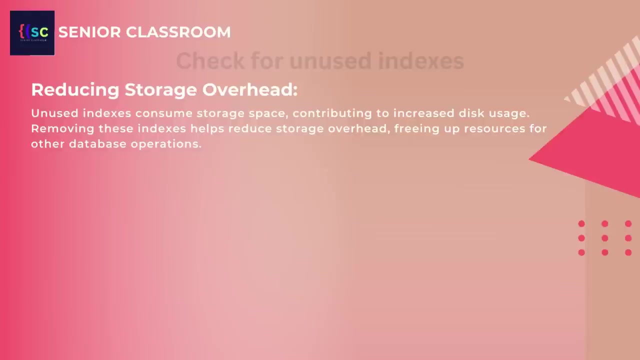 Regularly assessing and removing these unused indexes is a crucial optimization technique that helps maintain a lean and efficient database structure. Key considerations are Reducing storage. over time, Unused indexes Consume storage space, contributing to increased disk usage. Removing these indexes helps reduce storage overhead. 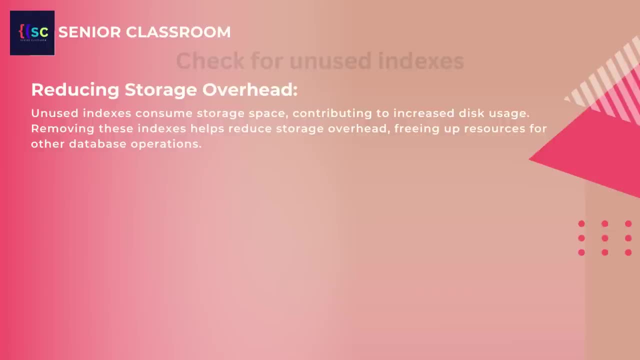 freeing up resources for other database operations. Improving write performance. Indexes incur maintenance costs during data modifications. inserts, updates, deletes Unused indexes. add to this overhead without providing corresponding benefits potentially impacting write performance. Enhancing query performance. Focusing on relevant indexes ensures that the query planner makes optimal decisions. 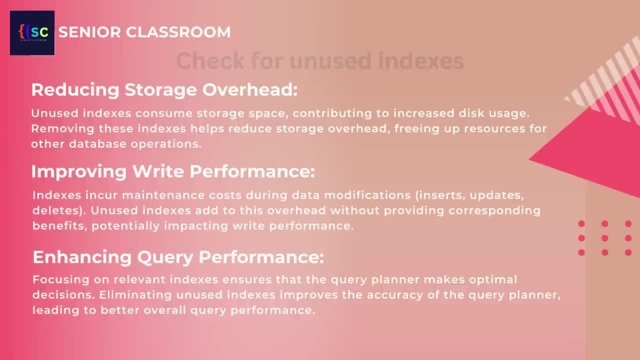 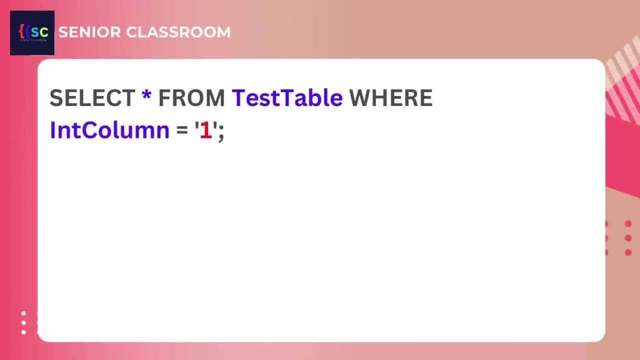 Eliminating unused indexes improves the accuracy of the query planner, leading to better overall query performance. Let's consider the following query. During the execution of this query, SQL Server will perform implicit data type conversion, converting int data to varchar before comparing. In such cases, indexes won't be utilized. 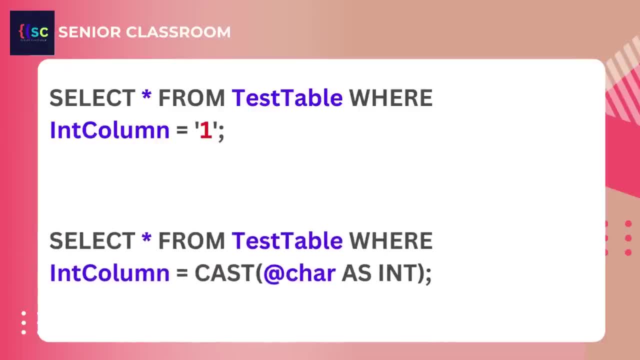 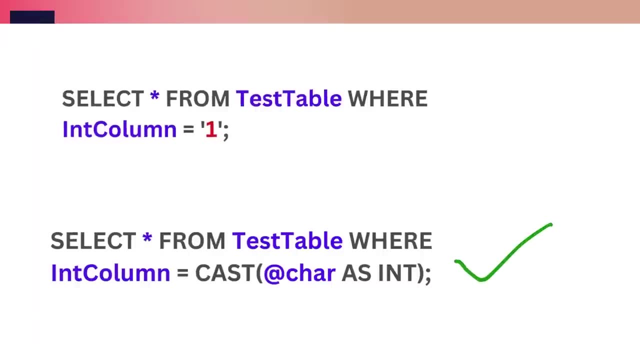 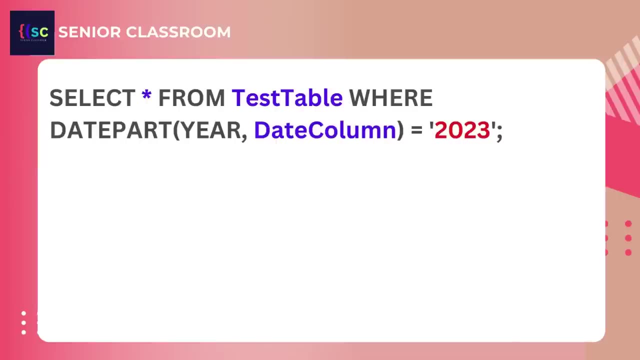 How can this be avoided? We recommend using the cast function, which converts a value of any type into a specified data type. Let's explore another example. In this scenario, implicit data type conversion will occur and the indexes won't be utilized. 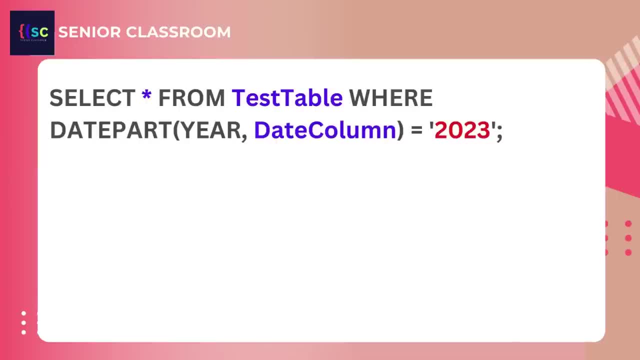 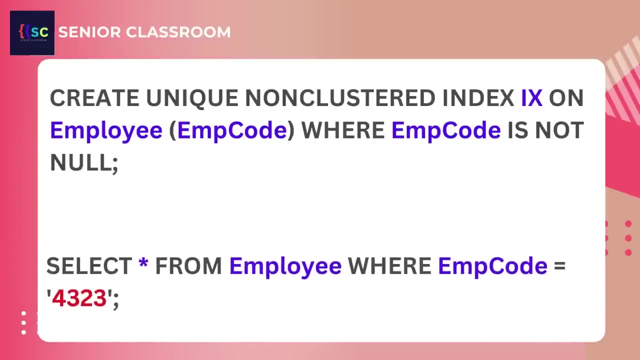 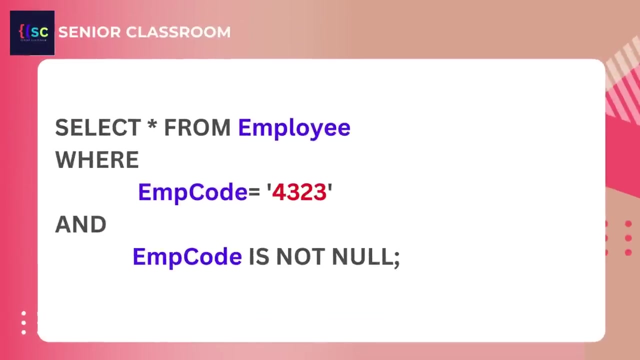 To address this, we can optimize the query as follows. Filtered indexes can impact performance as well. Consider having an index on the employee table. However, this index won't function as intended for the following query. To leverage the index, optimize the query in the following manner. 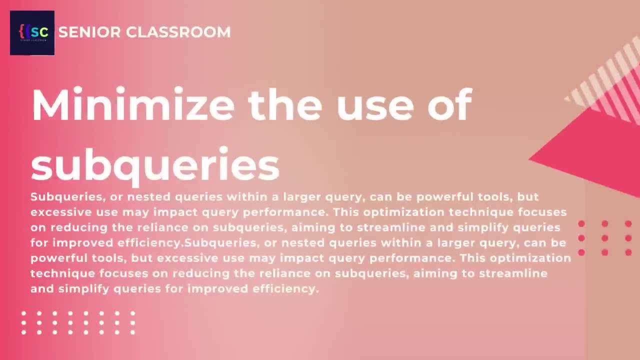 Minimize the use of subqueries. Subqueries or nested queries within a larger query can be powerful tools, but excessive use may impact query performance. This optimization technique focuses on reducing the reliance on subqueries, aiming to streamline and simplify query performance. 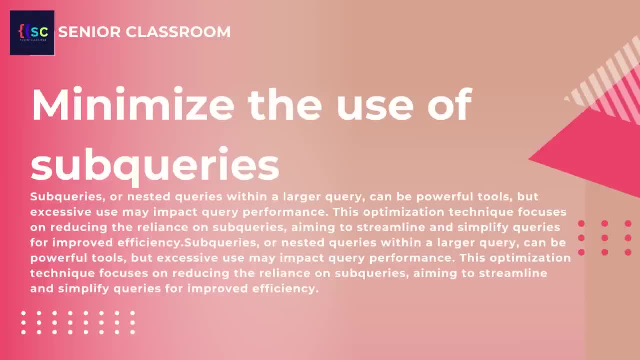 This optimization technique focuses on reducing the reliance on subqueries, aiming to streamline and simplify query performance. To leverage the index, evaluate the query structure. review your queries to determine how来 can they be achieved and how can they be applied to the query structure. 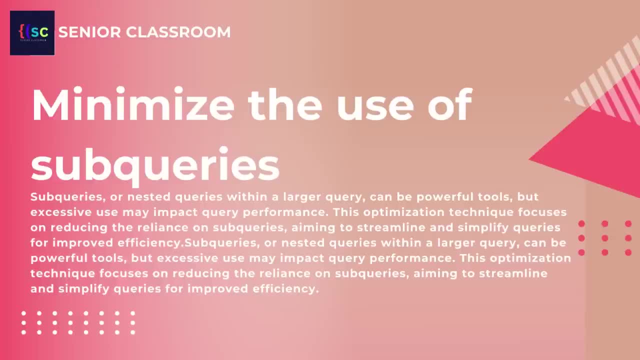 If the index means that the index is more than one item, you can reflect the indexes using the subqueries To understand how to apply the index, evaluate the index structure and analyze the index on the subqueries. The index can be used to evaluate the index of an individual user. 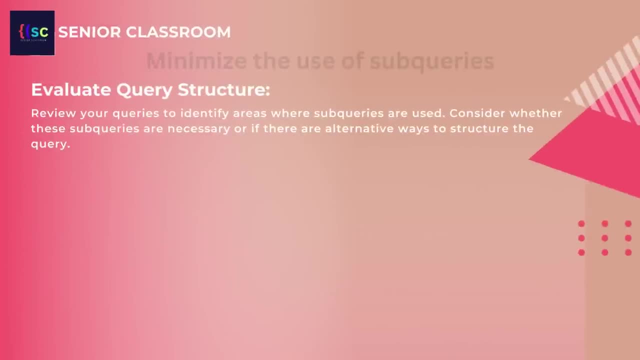 To show the index level of the index. you can pause the equation to see how a text is unstoppable. This is exactly what it is. You can view the index as an integral item of the index to identify areas where subqueries are used. 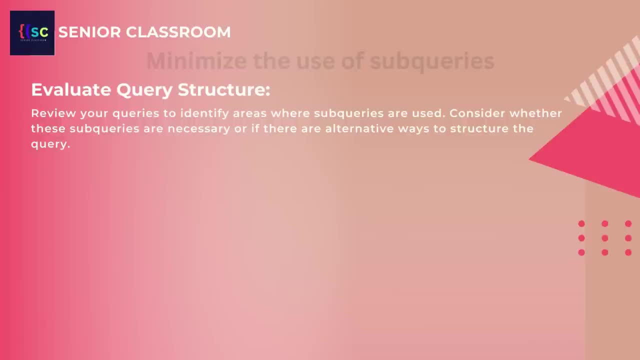 Consider whether these subqueries are necessary or if there are alternative ways to structure the query. Use joins or derived tables. Where possible, replace subqueries with join operations or derived tables. This can lead to more efficient execution plans. Optimize where clauses. 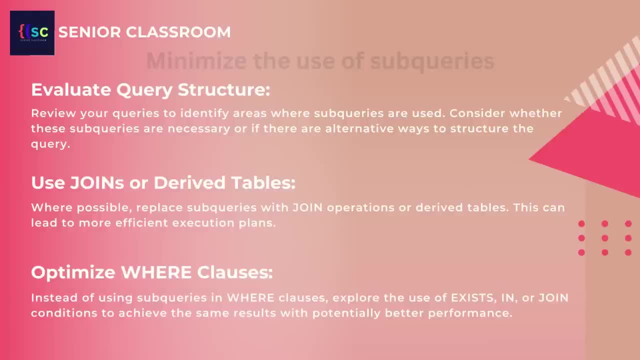 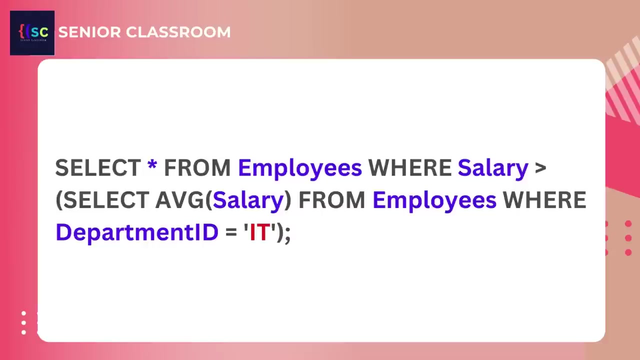 Instead of using subqueries in where clauses explore the use of, exists in or join conditions to achieve the same results with potentially better performance. Example: consider a query with a subquery to find the average salary of employees in a specific department. 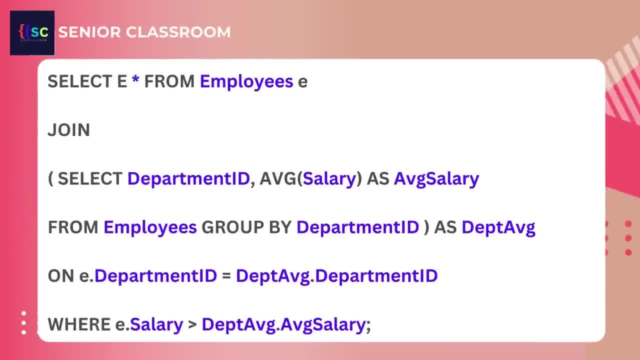 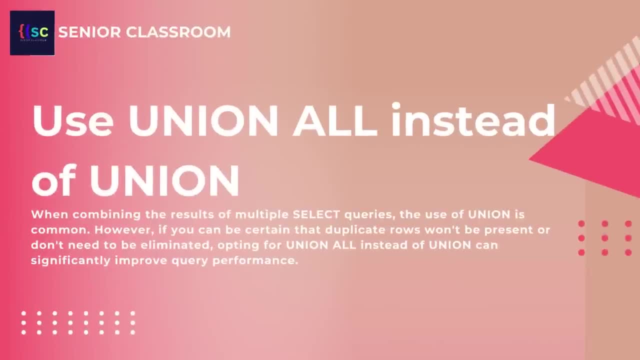 Optimize the query using a join. Next is use union all instead of union. When combining the results of multiple select queries, the use of union is common, However, if you can be certain that duplicate rows won't be present or don't need to be eliminated. 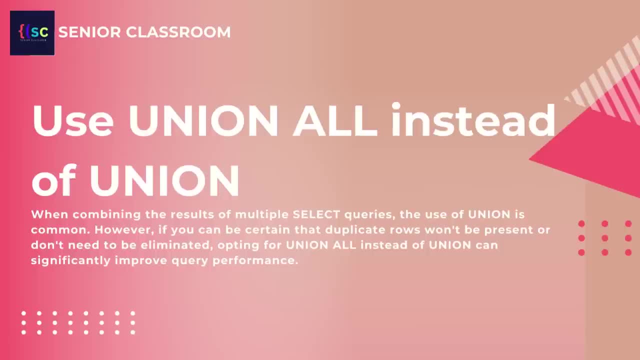 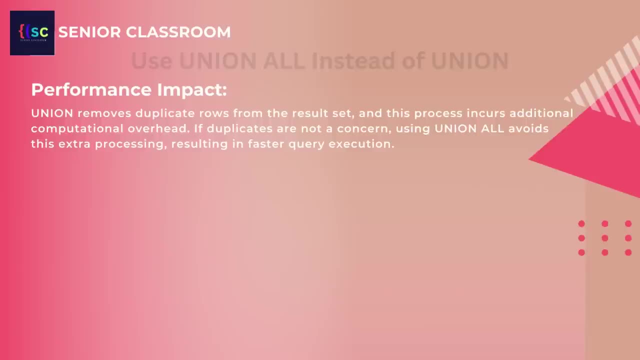 opting for union All instead of union can significantly improve query performance. Key considerations are: performance impact: union removes duplicate rows from the result set, and this process incurs additional computational overhead. If duplicates are not a concern, using union all avoids this extra processing. 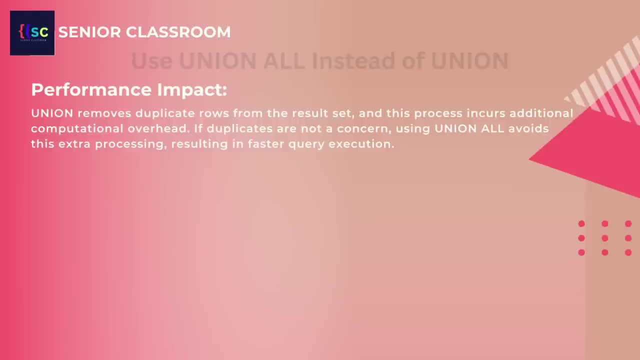 resulting in faster query execution. Reduced resource usage: Union all is more efficient in terms of resource usage as it doesn't require the database engine to perform the additional step of identifying and eliminating duplicate rows. Scenarios. Use union when you specifically need to eliminate. 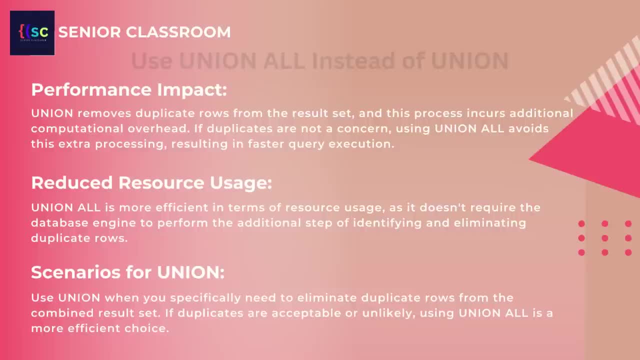 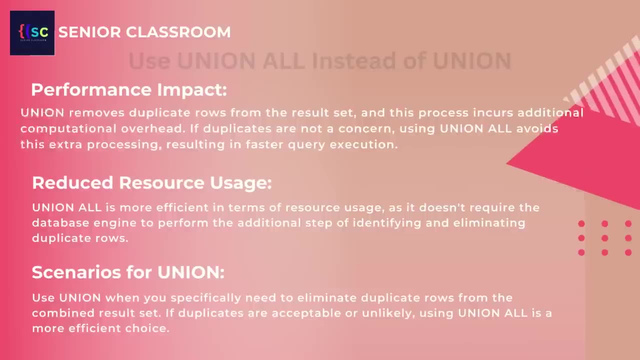 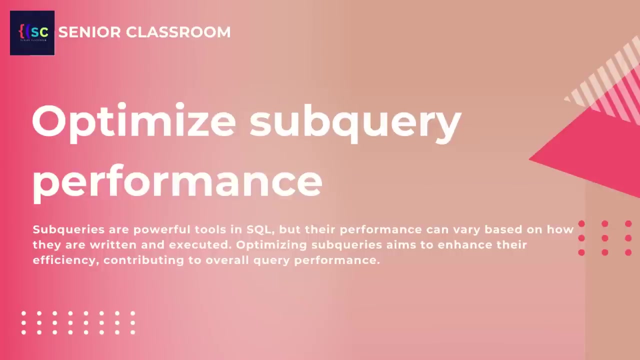 duplicate rows from the combined result set. If duplicates are acceptable or unlikely, using union all is a more efficient choice. Next is optimize subquery performance. Subqueries are powerful tools in SQL, but their performance can vary based on how they are written and executed. 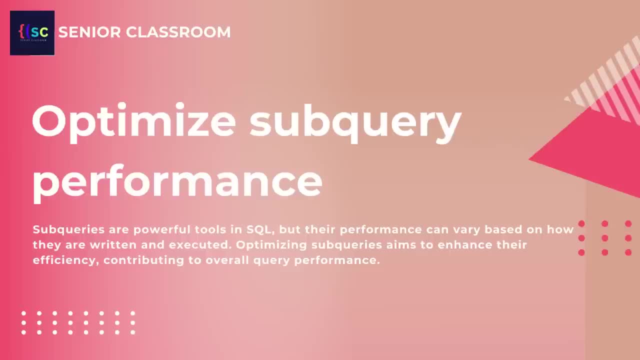 Optimizing subqueries aims to enhance their efficiency, but also to improve their performance. This is important for the performance of SQL, but also to improve the performance of SQL. This is important for the performance of SQL, but also to improve the performance of SQL. 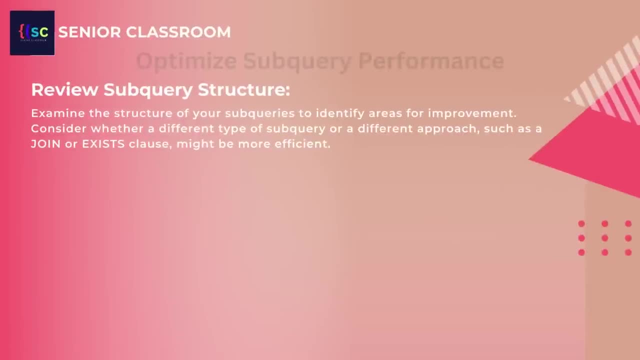 How to apply this technique. Review subquery structure. Examine the structure of your subqueries to identify areas for improvement. Consider whether a different type of subquery or a different approach, such as a join or exists clause, might be more efficient. 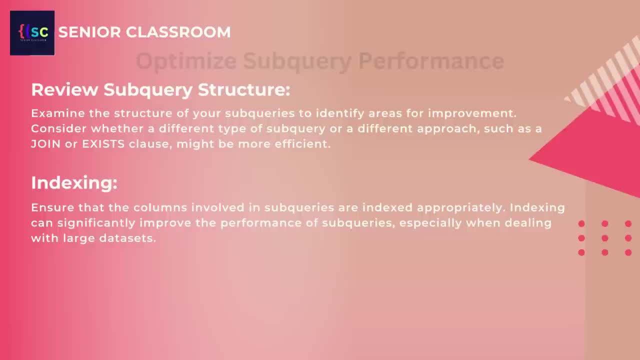 Indexing. Ensure that the columns involved in subqueries are indexed appropriately. Indexing Can significantly improve the performance of subqueries, especially when dealing with large data sets. Limit subquery results If possible. limit the number of rows processed by subqueries. 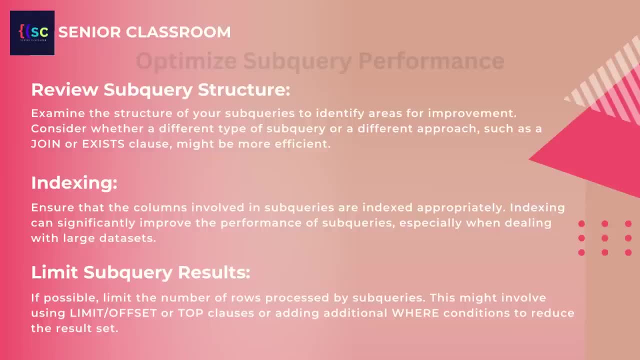 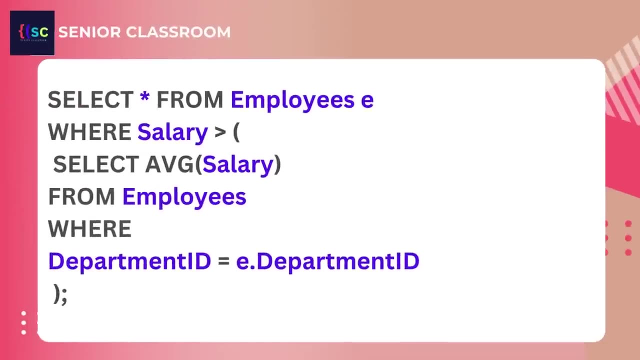 This might involve using limit, offset or top clauses, or adding additional where conditions to reduce the result set. Example: Consider a correlated subquery to find employees with salaries above the average for their department. Determine the subquery's performance. Optimize the query using a join. 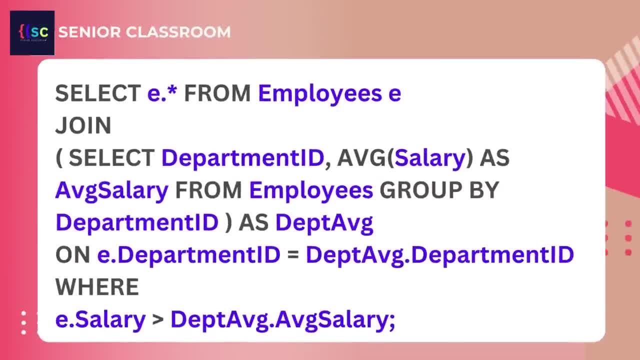 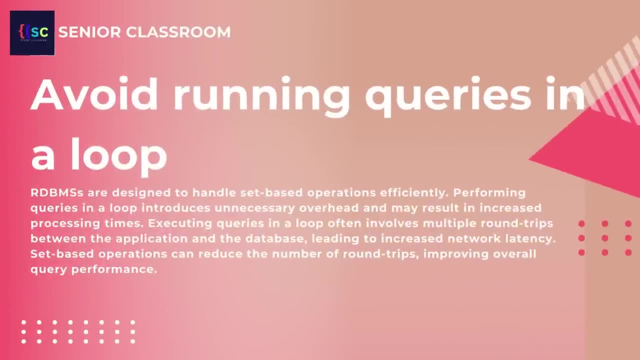 to achieve the same result more efficiently. Determine the subquery's performance. The optimization approach may vary based on the specific characteristics of your data and the database management system you are using. Determine the subquery's performance. Next is avoid running queries in a loop. 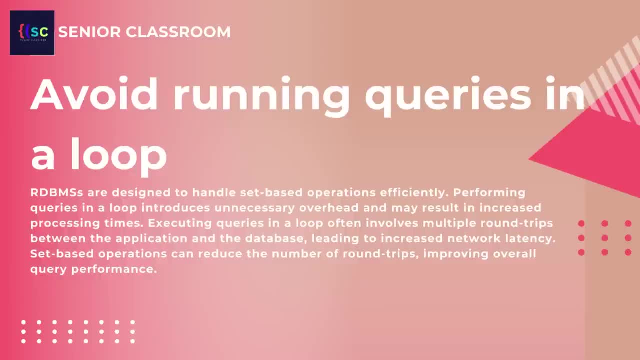 RDBMS says are designed to handle set-based operations efficiently Determine the subquery's performance. Performing queries in a loop introduces unnecessary overhead and may result in increased processing times. Executing queries in a loop often involves multiple round trips between the application and the database. 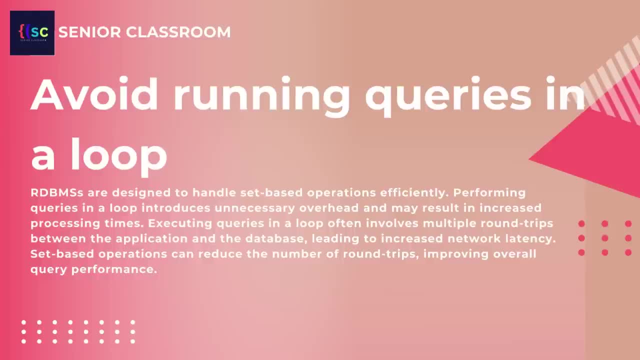 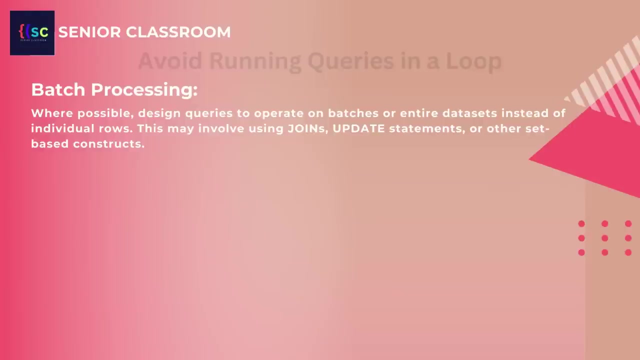 leading to increased network latency. Set-based operations can reduce the number of round trips, improving overall query performance. How to apply this technique: Batch processing, Where possible. design queries to operate on batches or entire datasets instead of individual rows. This may involve using joins. update statements. 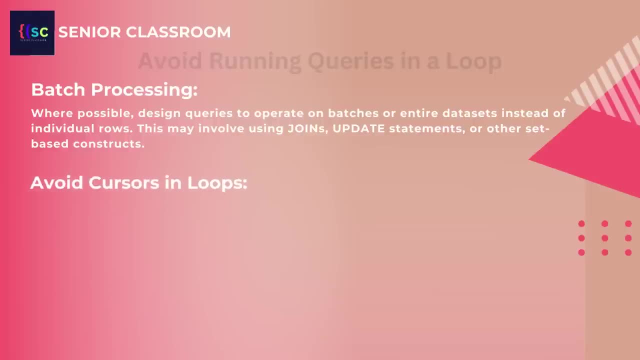 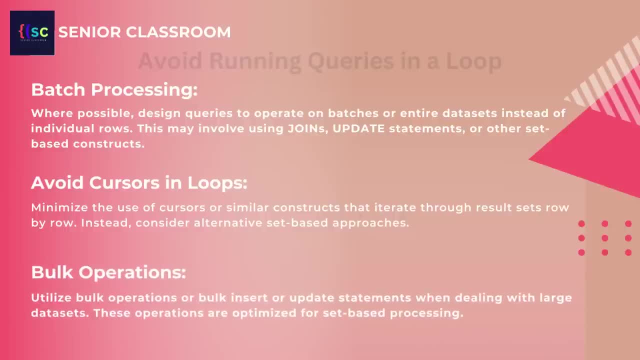 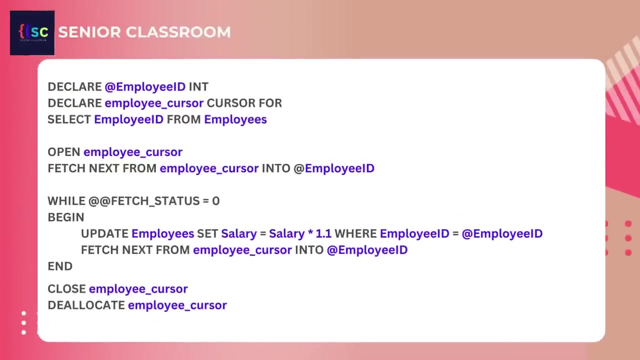 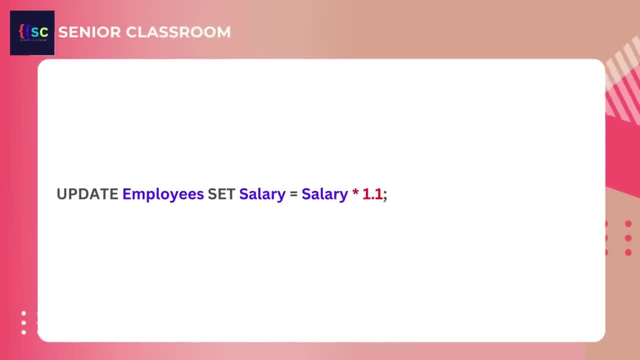 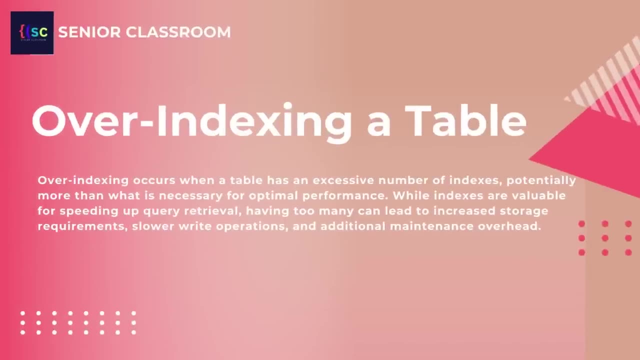 Optimize the update operation using a set-based approach. next optimization technique is avoid over indexing. a table over indexing occurs when a table has an excessive number of indexes, potentially more than what is necessary for optimal performance. while indexes are valuable for speeding up query retrieval, having too many can lead to increased. 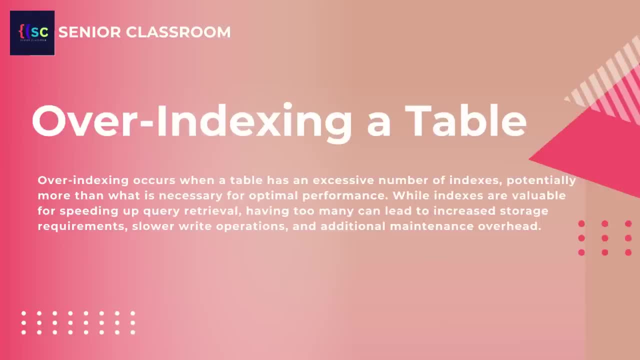 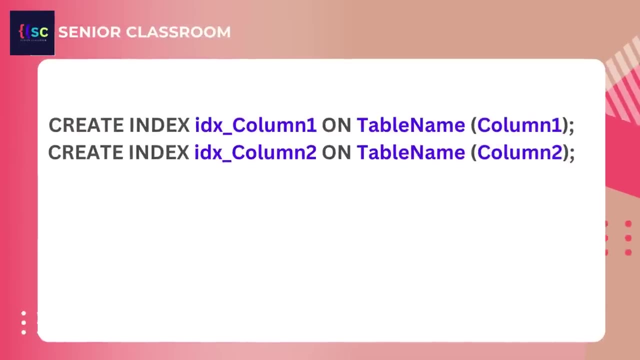 storage requirements, slower write operations and additional maintenance overhead. example: consider a scenario where a table has individual indexes on columns column 1 and column 2. optimize by using a composite index. the decision to create an index should be based on the specific query patterns and requirements of the application. next is use appropriate. 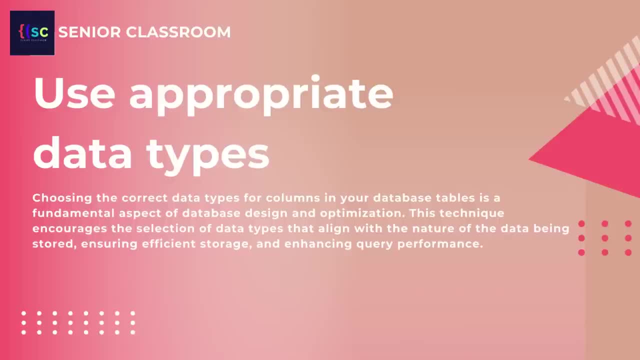 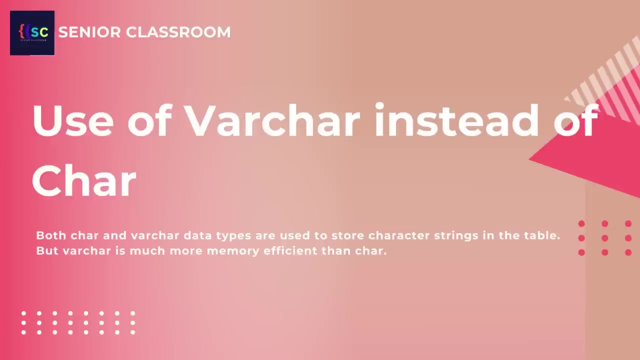 data types. choosing the correct data types for columns in your database tables is a fundamental aspect of database design and optimization. this technique encourages the selection of data types that align with the nature of the data being stored, ensuring efficient storage and enhancing query performance. next optimization technique is use VAR char instead of char when defined. 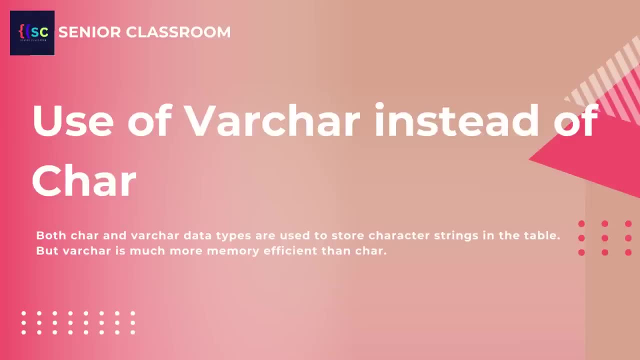 character columns in a database table. selecting between VAR, char and char depends on the nature of the data. this optimization technique encourages the use of VAR char for variable length character data when the length of the stored values varies, optimizing storage space and improving overall performance. char columns allocate a fixed amount of storage space for each value padding shorter. 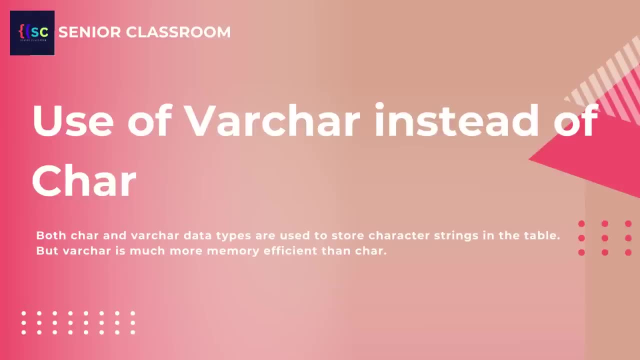 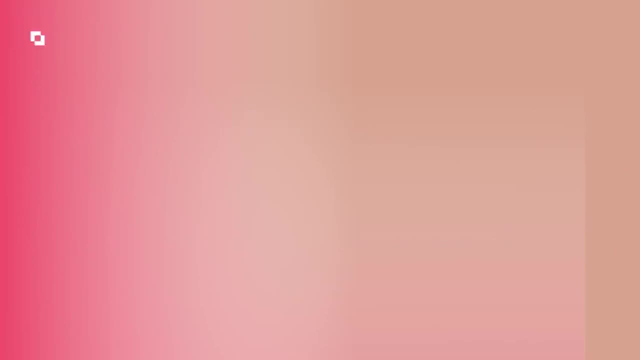 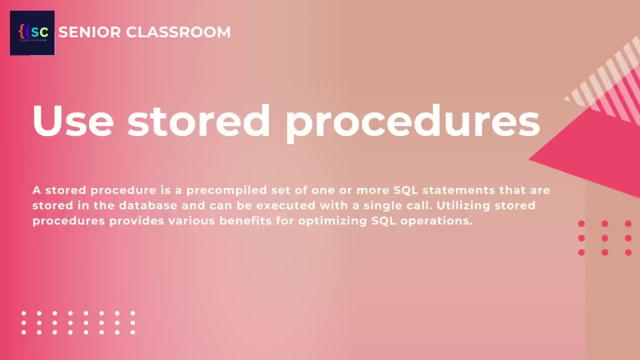 values with trailing spaces. in contrast, VAR char columns only store the actual length of the value, leading to more efficient storage. next optimization technique: use stored procedures. a stored procedure is a pre-compiled set of one or more SQL statements that are stored in the database and can be executed with a single. 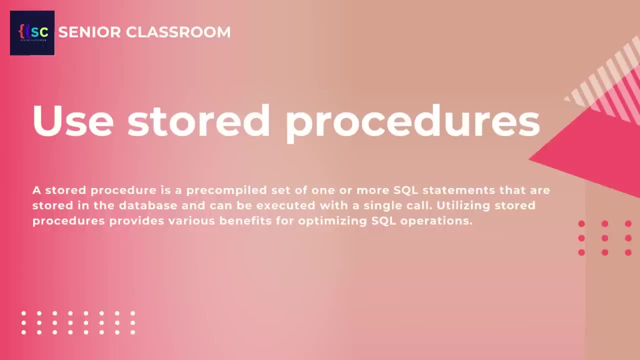 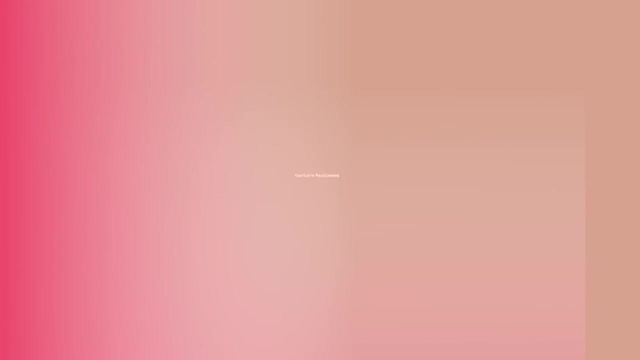 call. utilizing stored procedures provides various benefits for optimizing SQL operations. stored procedures are executed on the database server, reducing the amount of data that needs to be transmitted between the database and the application. this can significantly minimize network traffic, especially for complex operations. stored procedures promote code reusability, since the same logic can be invoked from multiple parts of the application. this can lead to a more modular and maintainable codebase. stored procedures are executed on the database server, reducing the amount of data that needs to be transmitted between the database and the application. this can significantly minimize network traffic, especially for complex operations. stored procedures promote code reusability, since the same logic can be invoked from multiple parts of the application. this can lead to a more modular and maintainable codebase. stored procedures are executed on the database server, reducing the amount of data that needs to be transmitted between the database and the application. this can significantly minimize network traffic, especially for complex operations. stored procedures promote code reusability, since the same logic can be invoked from multiple parts of the application. this can lead to a more modular and maintainable codebase. stored procedures are executed on the database server, reducing the amount of data that needs to be transmitted between the database and the application. 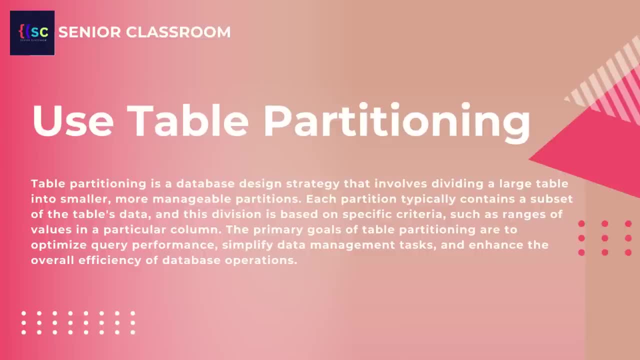 next optimization technique is table partitioning. table partitioning is a database design strategy that involves dividing a large table into smaller, more manageable partitions. each partition typically contains a subset of the table's data, and this division is based on specific criteria, such as ranges of values in a particular column. the primary goals of table partitioning are to optimize query performance, simplify data management. 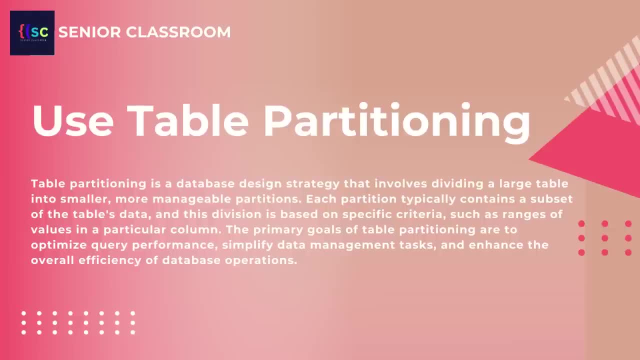 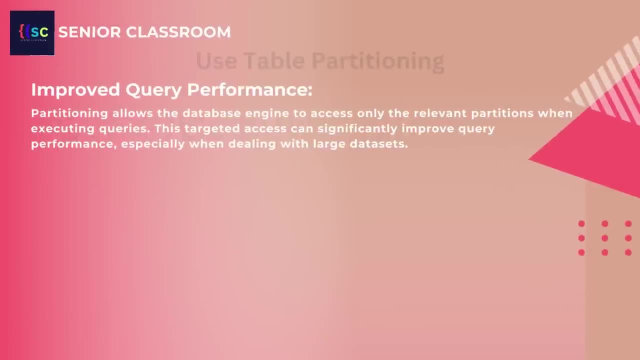 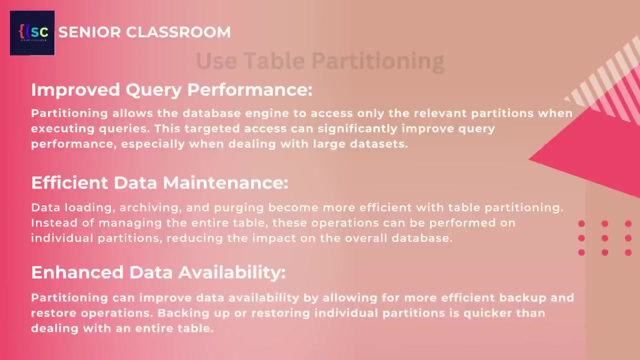 tasks and enhance the overall efficiency of database operations. key considerations: improved query performance: partitioning allows the database engine to access only the relevant partitions when executing queries. this targeted access can significantly improve query performance, especially when dealing with large data sets. efficient data maintenance, data loading and archiving and purging become more efficient with table partitioning. instead of managing the entire table, these operations can be performed on individual partitions, reducing the impact on the overall database. enhanced data availability: partitioning can improve data availability by allowing for more efficient backup and restore operations. backing up or restoring individual partitions is critical to the 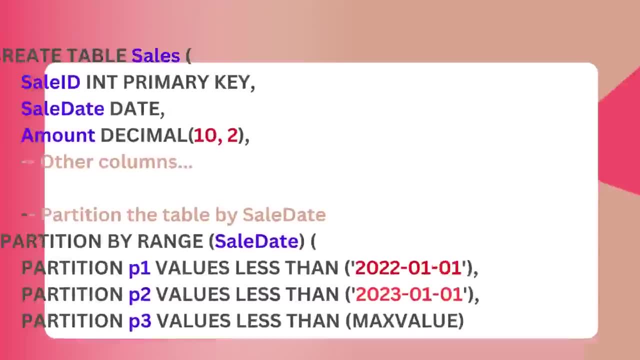 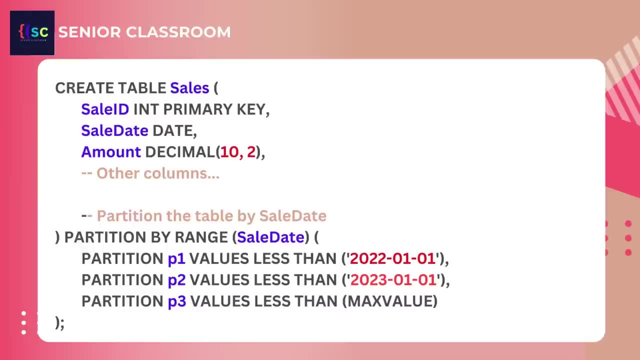 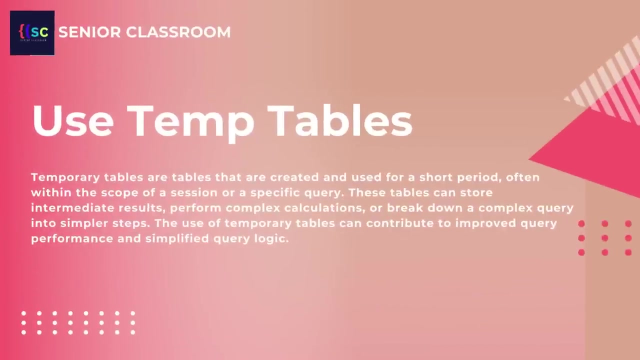 quicker than dealing with an entire table. for example, consider partitioning a large sales table by date ranges. the exact syntax and capabilities for table partitioning may vary depending on the database management system. next optimization technique is use temporary tables. temporary tables are tables that are created and used for a short period. 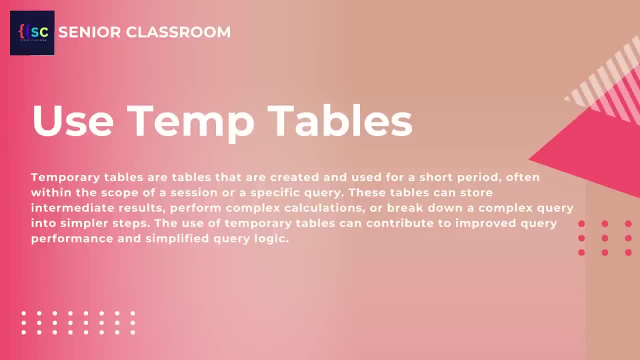 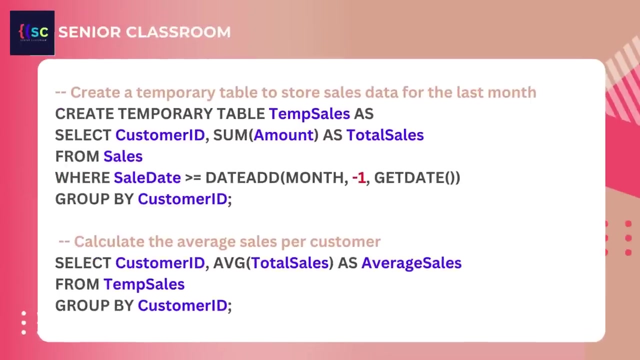 often within the scope of a session or a specific query. these tables can store intermediate results, perform complex calculations or break down a complex query into simpler steps. the use of temporary tables can contribute to improved query performance and simplified query logic. consider a scenario where you need to calculate the average sales per customer for the last month. 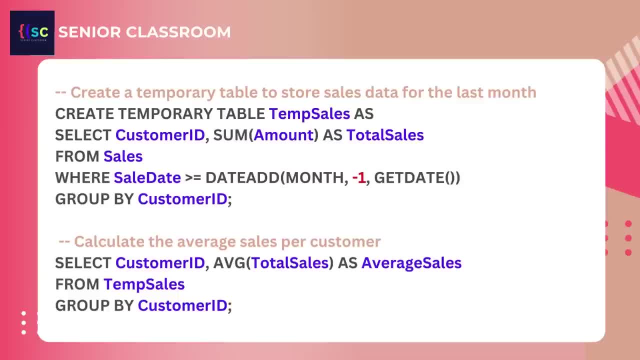 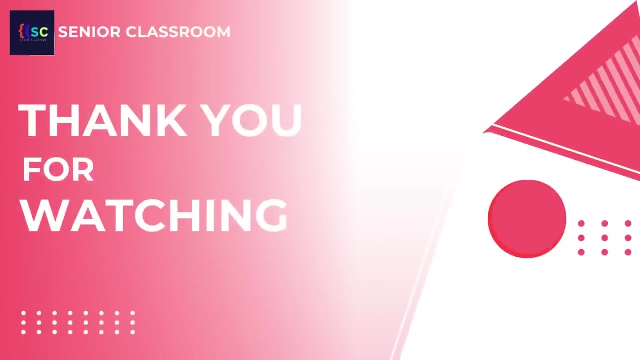 using a temporary table can simplify the process. by using temporary tables, you can streamline complex query operations, improve performance and simplify the overall logic of your SQL queries, especially when dealing with multistep or intricate data manipulations. and that brings us to the end of our video on optimizing SQL queries we've covered. 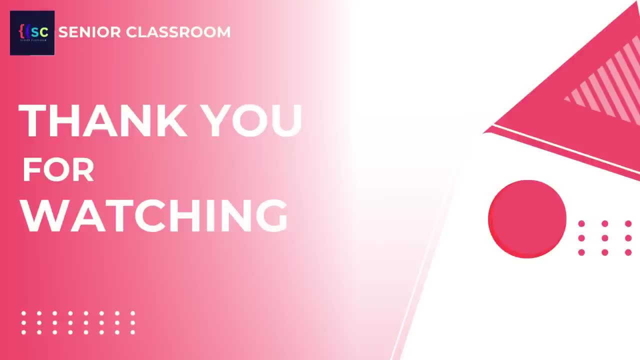 essential techniques, highlighting the importance of streamlining your code for efficient database performance. If you found these insights valuable, don't forget to hit the like button, subscribe for more content and share this video with your fellow developers. Your support means a lot. Happy querying and I'll catch you in the next one.